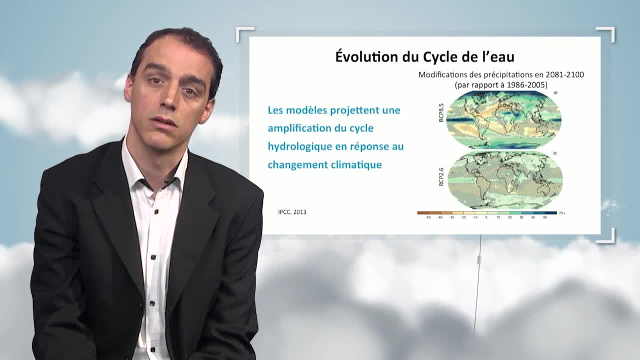 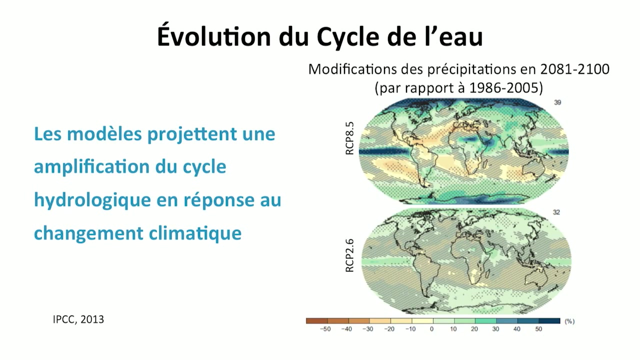 rain Climate models forecast: amplification of rain in wet areas and average latitudes in the equatorial belt and decreased rains in subtropical areas- dry areas. Two maps showing the two extreme scenarios: RCP 85, where gas emissions are substantial until. 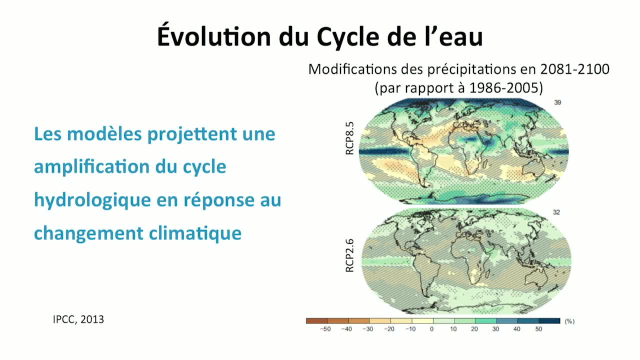 the end of the century, and RCP 2.6, where gas emissions are decreased. This is an example of the two extreme scenarios: RCP 85, where gas emissions are substantial until the end of the century, and RCP 2.6, where gas emissions are substantial until the end of. 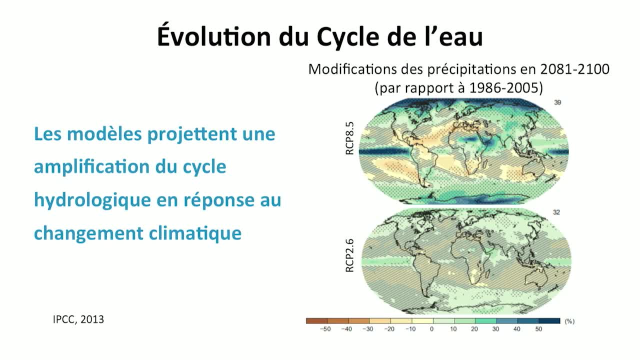 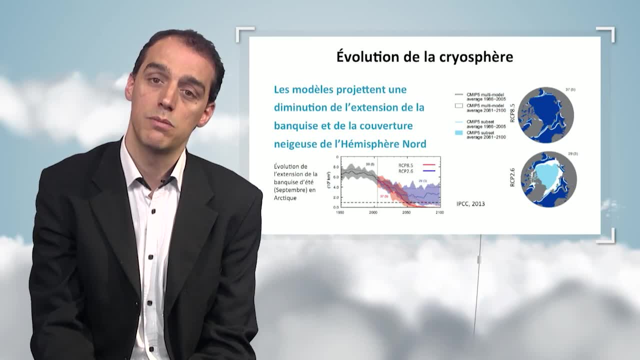 the century and RCP 2.6, where gas emissions are substantial, until the end of the century. Now changes in the rain distribution are more obvious in terms of amplification and reduction in the RCP 8.5 scenario. Second aspect of the climatic aspect: evolution in the cryosphere and the ice-covered areas. 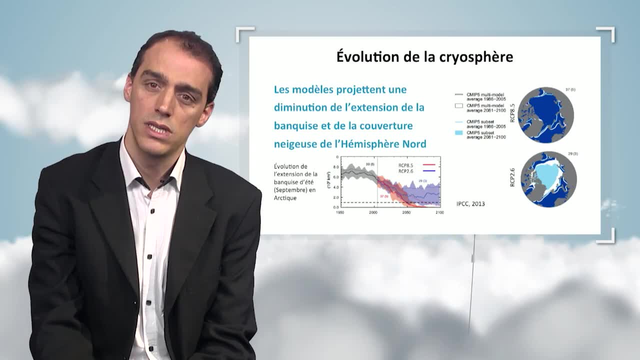 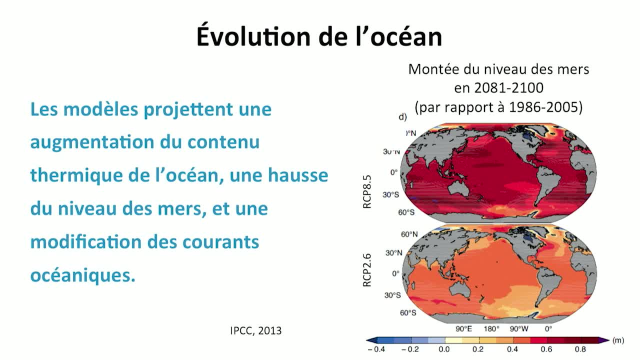 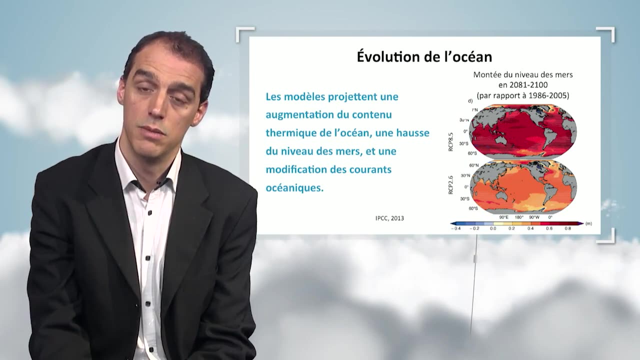 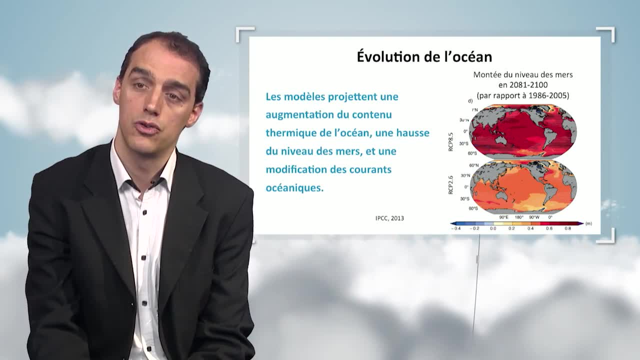 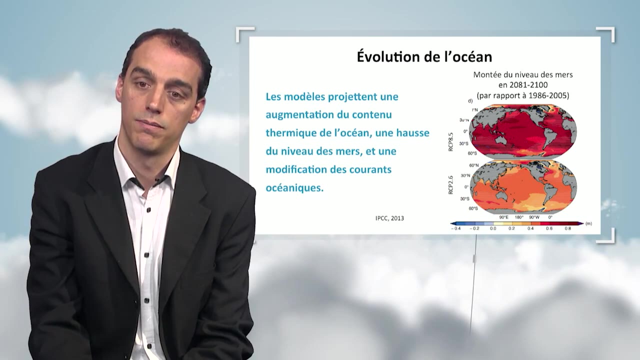 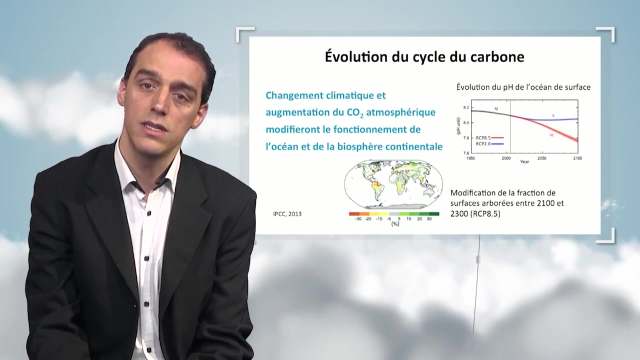 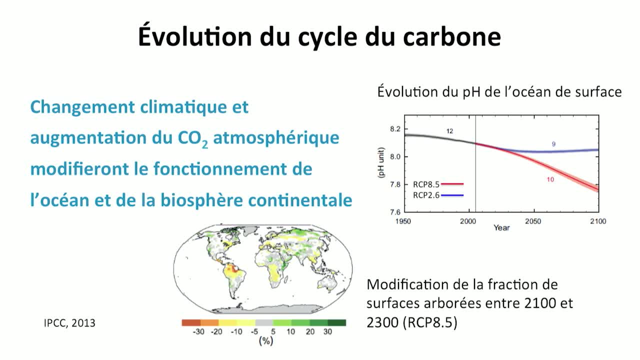 We see the carbon cycle in the natural reservoirs such as the ocean and the continental land. Two examples: on the right-hand side, pH evolution on the surface layer of the ocean. due to the fact that the ocean continues absorbing entropic carbon, CO2 is a low acid and therefore the ocean will lose several units of pH by the year 2100. 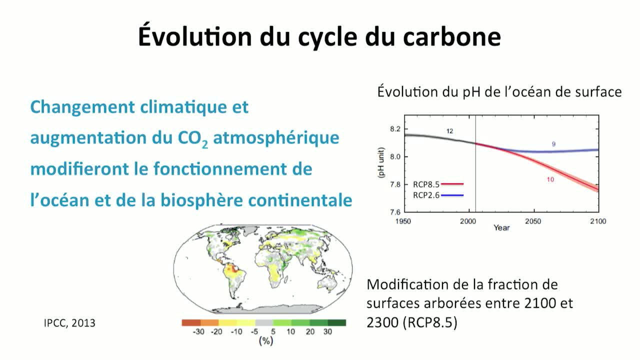 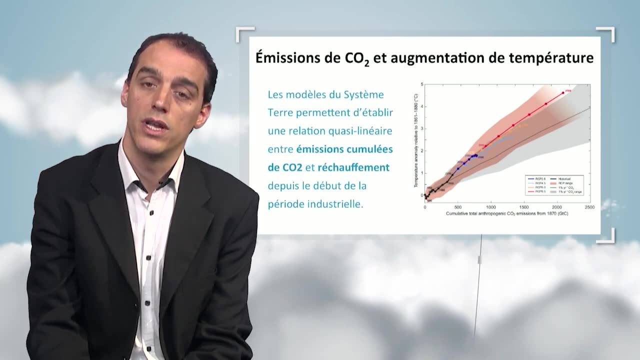 And on the bottom map we see the changes in the forest-covered areas in the world, with many changes due to climatic changes and the fact that some areas will become drier. Finally, thanks to simulation of the CO2 cycle, the carbon cycle will continue to grow.